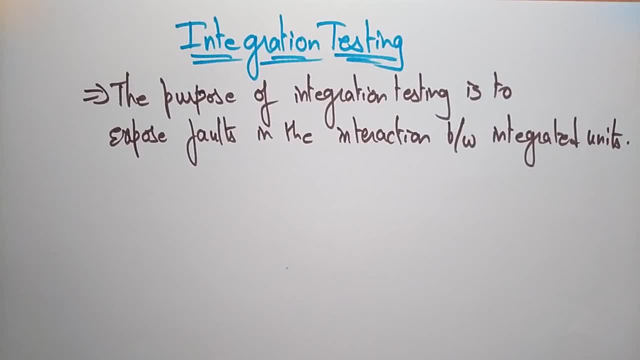 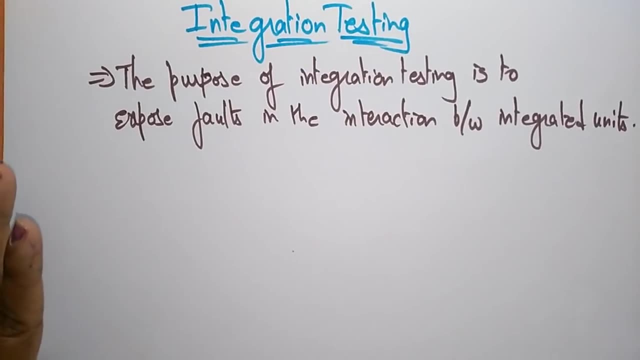 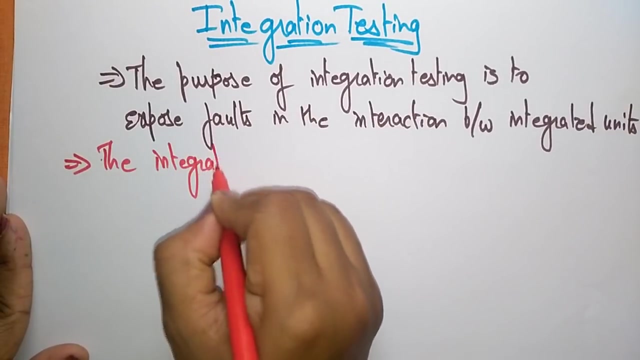 So you will get some faults. the faults will be raised So that you have to be tested by using integration testing. So the integration testing is a process of testing. Let me write the definition for that. The integration testing is the process of testing. 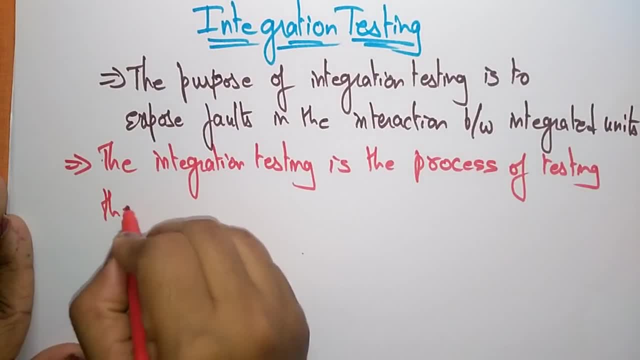 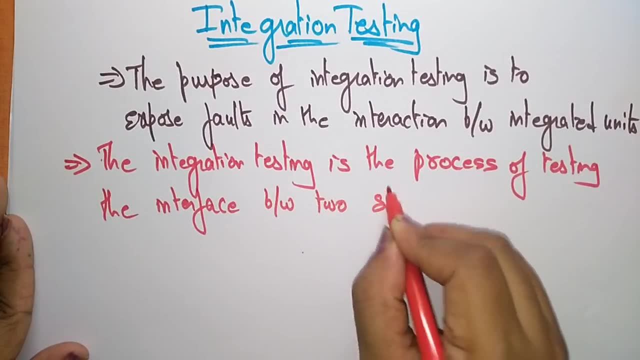 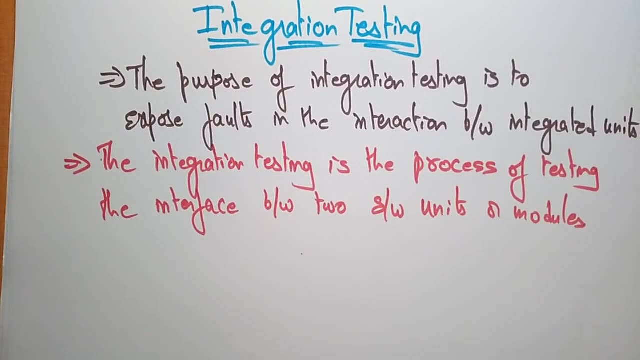 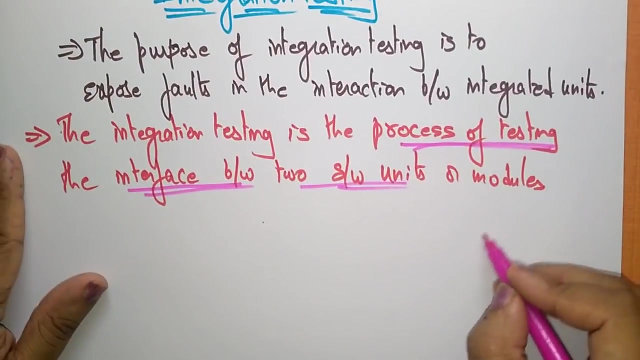 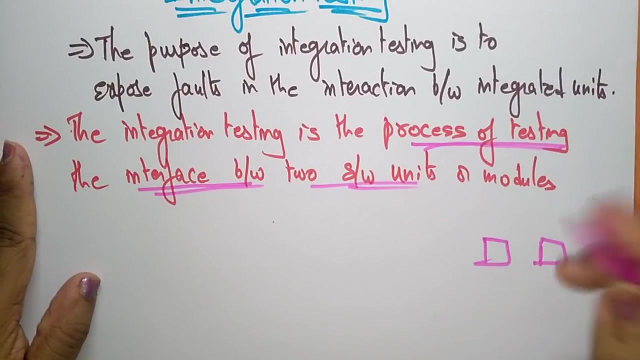 Is the process of testing The interface between, interface between two software units, two software units or modules. So what it is saying- integration testing- is nothing, but it is a process of testing. the interface between two software units Means here two software units are there. So the testing that is done on the interface between two software units. 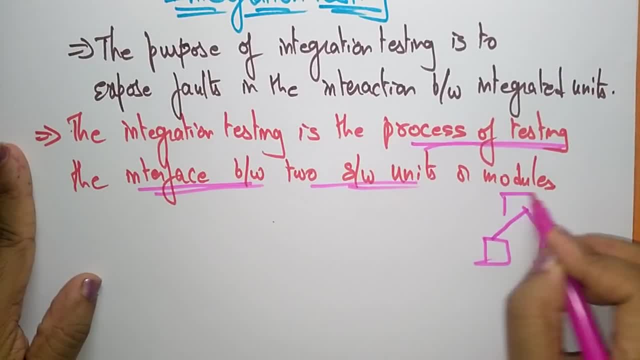 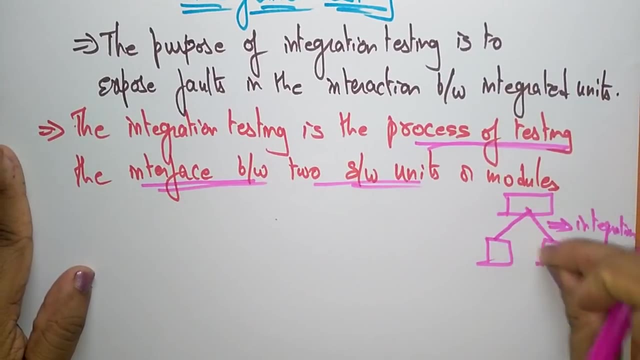 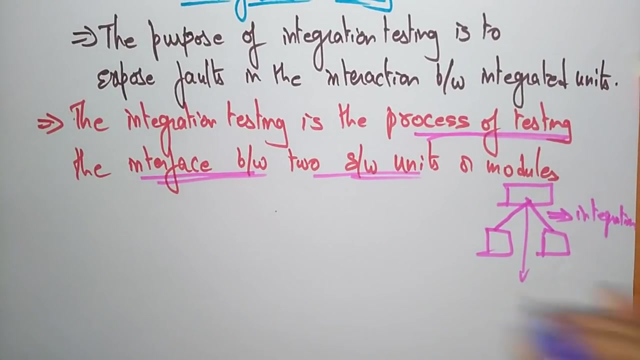 So this is interfacing, So this is interfacing and interfacing. These two interfacing units are combined and clubbed into one module. So here we are performing integration testing, The process of testing the interfaces between interfaces between two software units or modules. So integration testing can be done in three ways. 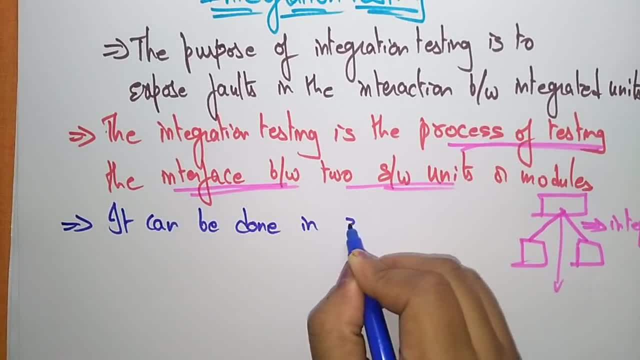 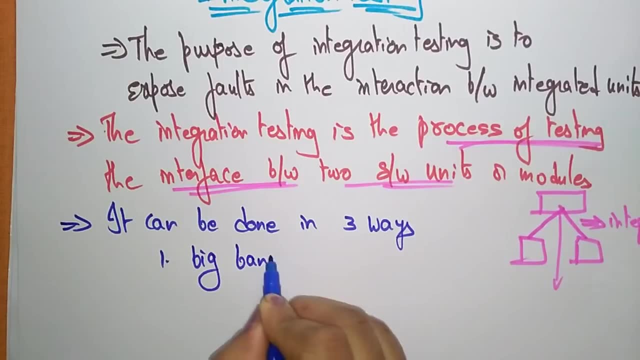 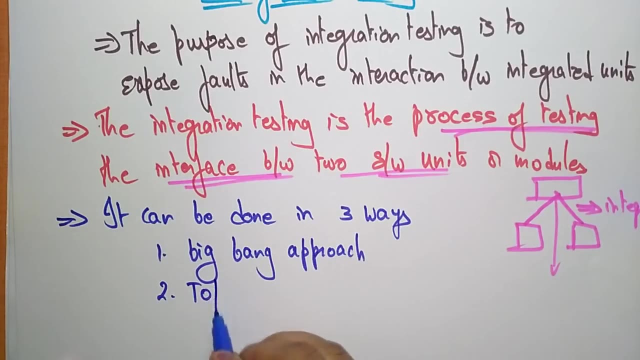 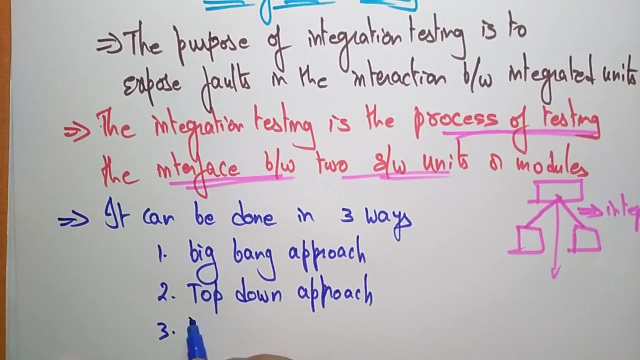 So integration testing can be done in three ways. So what are the three ways? The first one is big bang approach, Big bang approach. So again, top down approach, Top down approach. And the third one is bottom up approach. so these are the three ways of the three ways of integration testing. now let us see the first one. 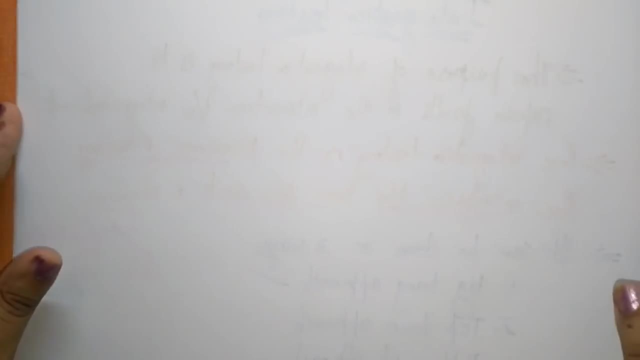 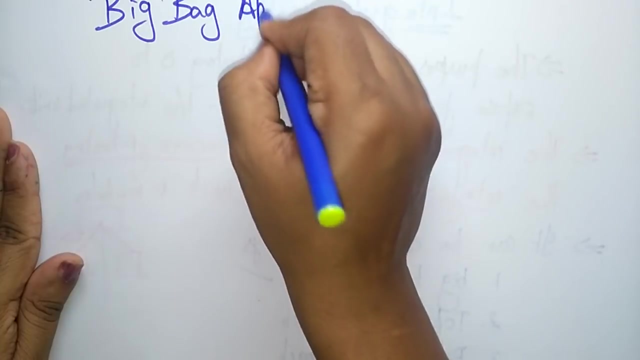 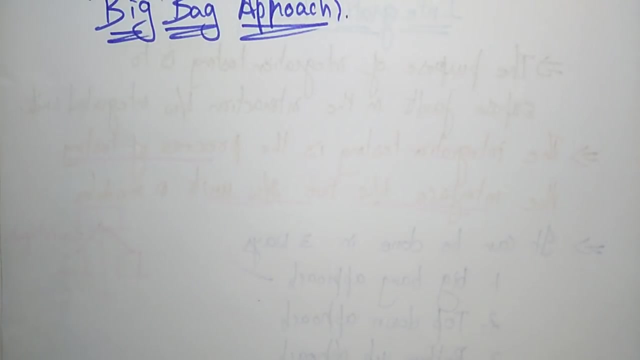 that is a big, big bang approach. so what is this big bang approach? so big bang approach is combining all the modules once and verifying the functionality after completion of individual module testing. so actually the integration testing is nothing, but we are just combining the modules and we are testing on that modules. 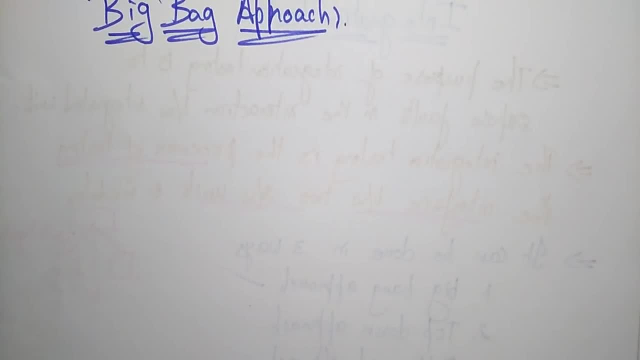 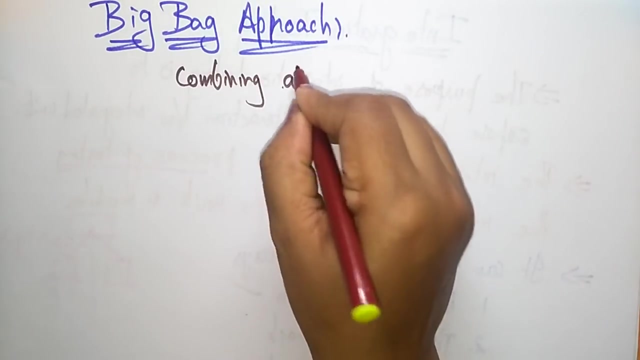 that is, the unit modules has to be. you know, the unit modules has to be, the unit modules has to be, the unit modules has to be integrated and tested. so that is integration testing. so one of the approach here is a big bang approach. so what this big bang approach is doing, it is combining, combining all the modules. 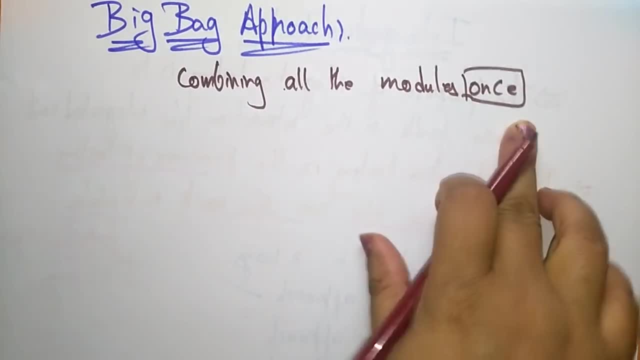 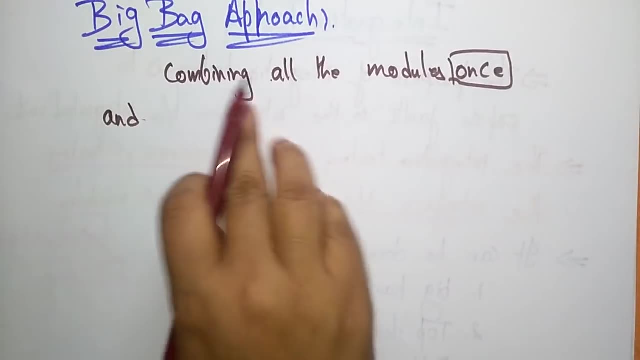 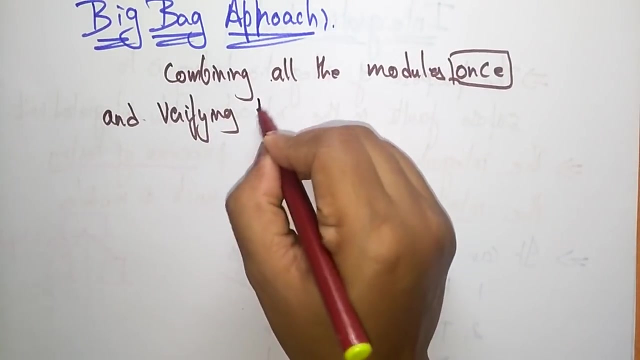 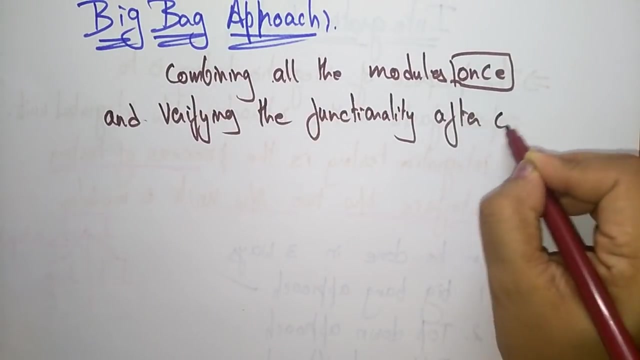 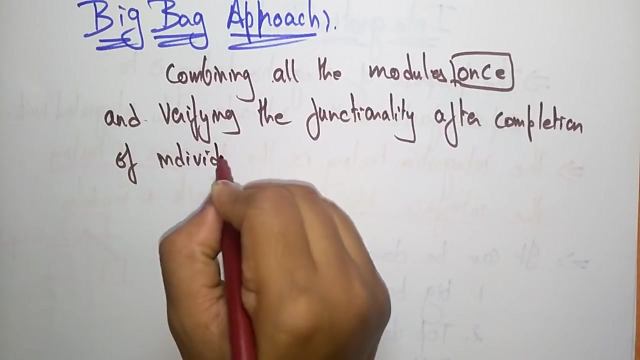 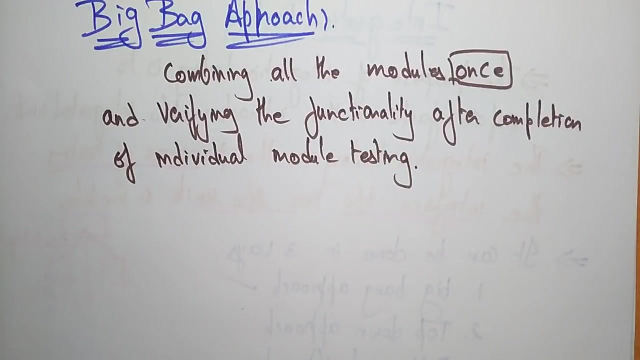 once. so this thing you have to be note down, all the modules once- and verifying, combining all the modules once and verifying the functionality after completion of individual module testing, individual module testing. so that is the big bang approach. so the main thing here, the big bang approach is you have to combine all the modules. 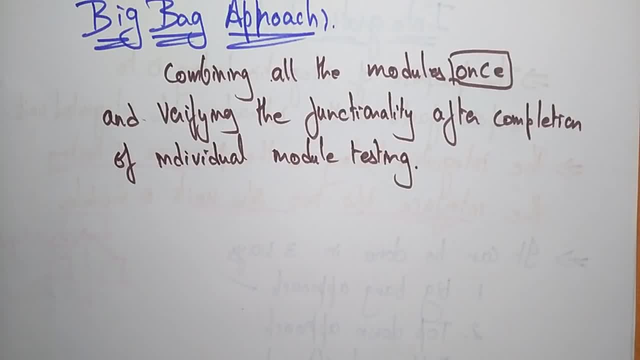 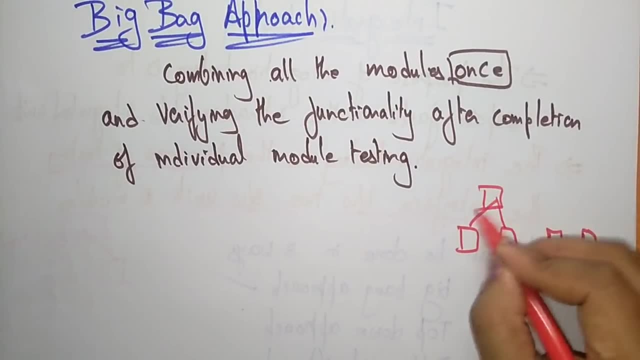 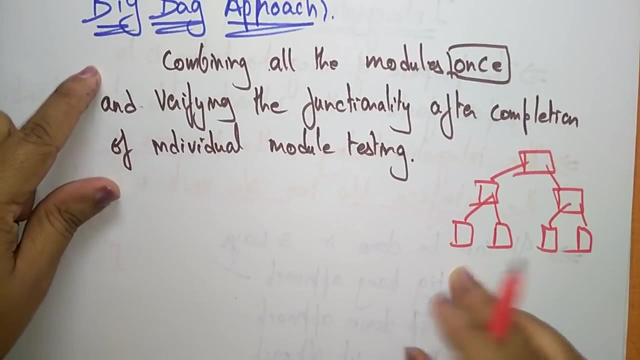 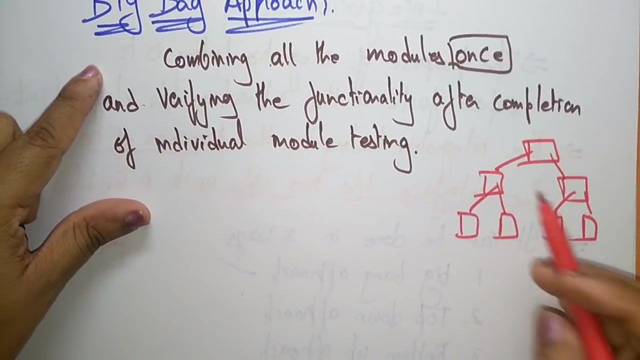 once and verify the functionality after the completion of individual model testing. so here a modules will be there, so these modules will be integrated again. this will be integrated, okay, so here the big bang approach is we have to combine all the modules once and verify the functionality when you are going to verify the functionality after the completion of the individual module test. 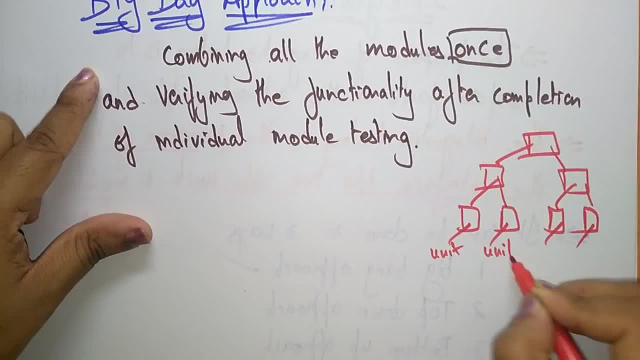 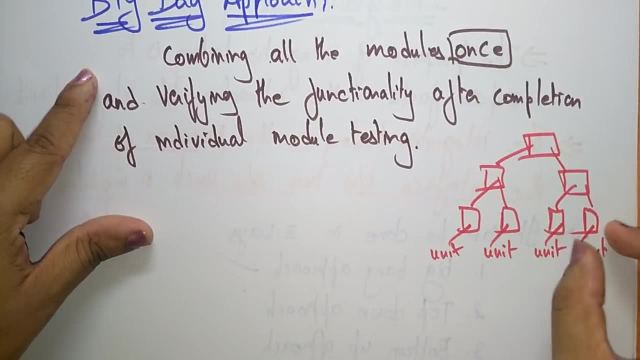 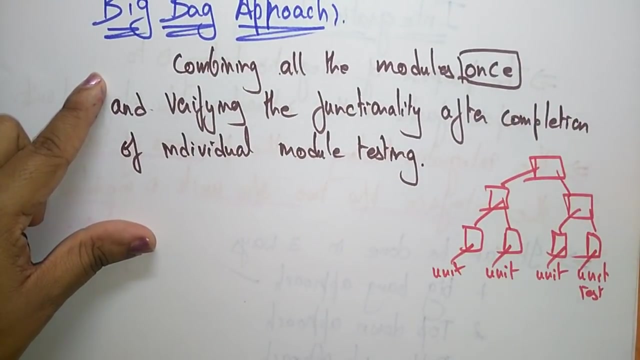 so this will be done on with the help of unit test. okay, so this will be done. the test will be done on this individual modules by with the help of unit test. so after completion of this individual module testing, you have to combine all the modules once and verify the functionality. then you have to. 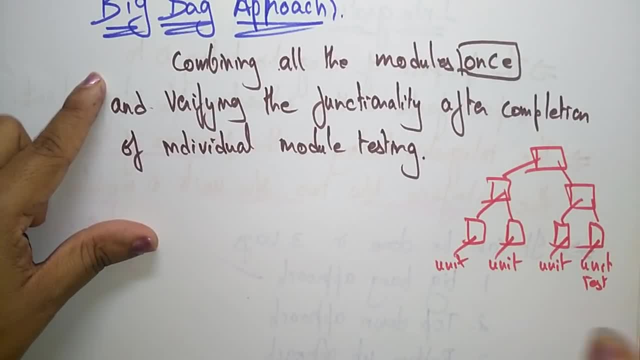 verify the functionality only after the completion of the individual module test. only. you have to verify the functionality means once here we are checking, even though we are checking by combining the two modules, again you have to check. so the checking done here is called integration testing. so this integrative testing we are done by using.